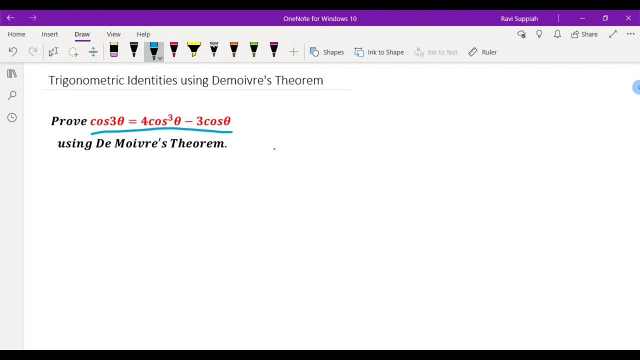 theorem first to see what we can observe. So in order for me to get cos 3 theta here, we know that the power n must be 3.. So just to quickly recap: what is Demogorgon's theorem when you have z to? 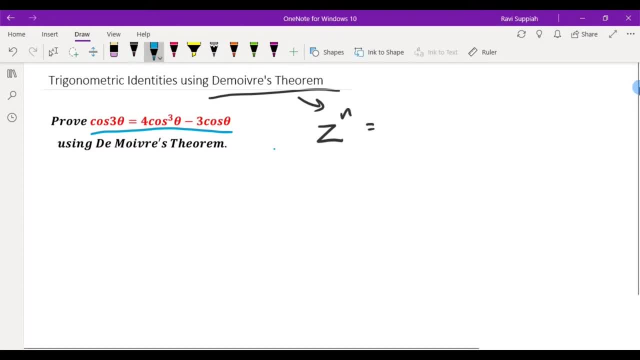 the power of n. okay, and z is a complex number, which is r cos theta plus j sin theta, the whole thing to the power of n. What Demogorgon's theorem says is this is equivalent to r to the power of n, into cos n theta plus j sin n theta, okay. 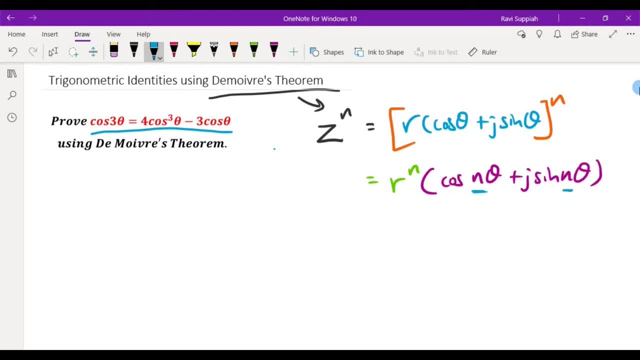 So, in order to do this observation, we can see that the n in this case is 3, okay, So n is equals to 3.. So we can now write: cos theta plus i sin theta to the power of 3 will be equals to. 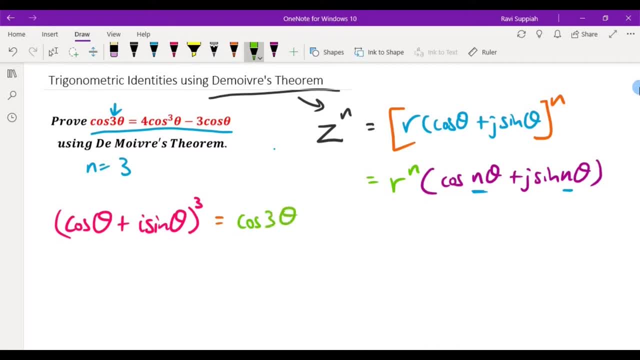 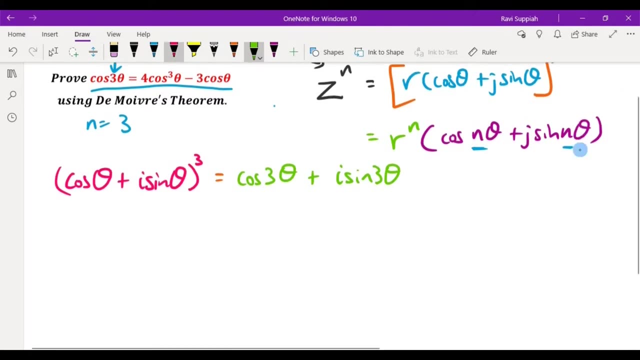 cos 3 theta plus i sin 3 theta. Okay Now. so this is the application of the Demogorgon's theorem. Now, what we're going to do now is to just see how this would expand if I were to just do it in the algebraic fashion. okay, 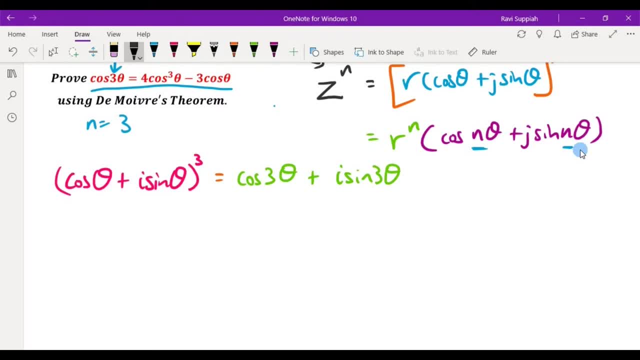 So, to make our analysis a bit easier, what I'm going to do is: I'm going to say that cos theta can be represented with x and i sin theta can be represented with x. So I'm going to say that cos theta can be represented with y, okay, So that is how we're going to proceed now. So this is. 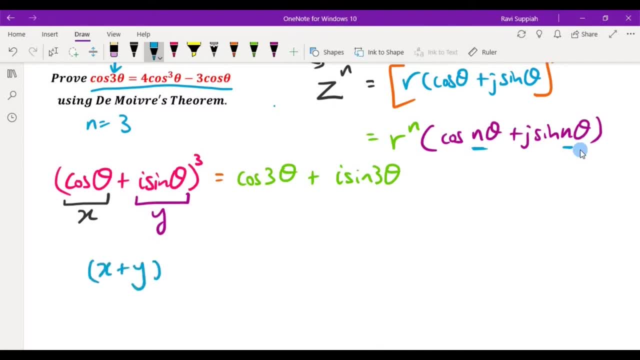 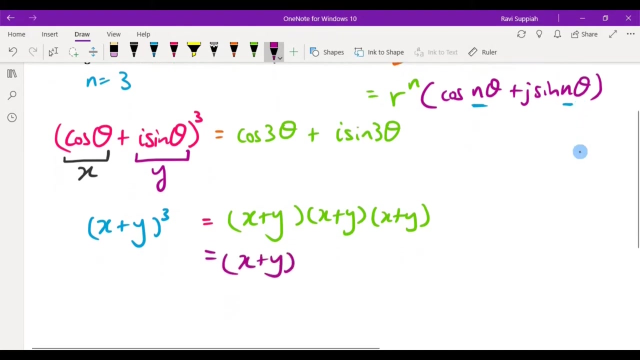 equivalent to writing x plus y cubed, and that is equals to x plus y multiplied into x plus y, into x plus y. Okay, So let's keep the first bracket and expand the second and third bracket using the normal expansion, the normal expansion approach. So what you will get over here is x squared plus. 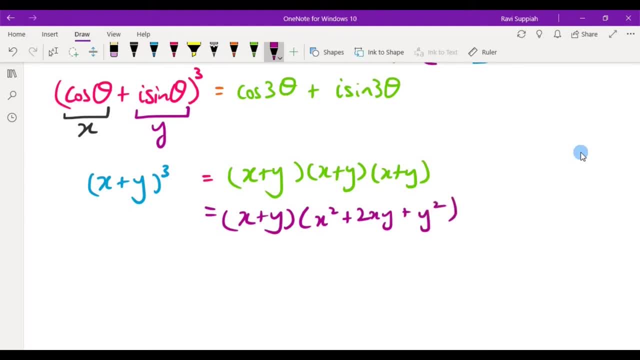 2xy plus y squared, okay, And then we can expand one more time over here. So x into x cubed, x into x squared, you get x cubed plus x into 2xy, you get 2x squared. y plus x into y squared is xy. 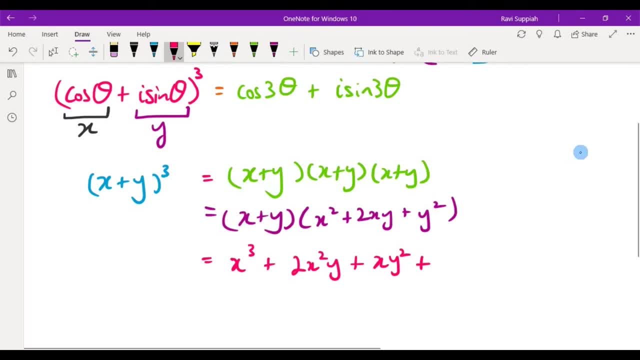 squared, okay. From the y, what you get is yx squared, yx squared, y into 2xy is plus 2xy squared, and y into y squared is plus y cubed. okay, And then you can group the similar terms together. So here, x cubed, you only. 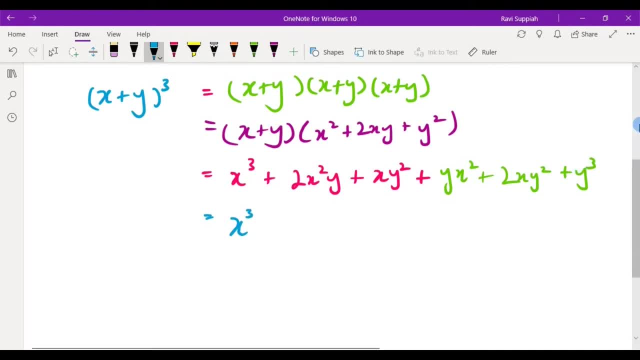 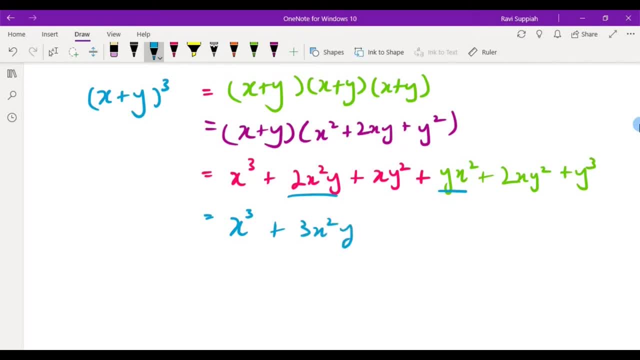 grouped together to get 3xy, xy squared, xy squared again. you have two of them, you can group them together to get 3xy squared And finally you have y cubed. Okay, Now taking this and now substituting it back in the back into the actual x and y representation. 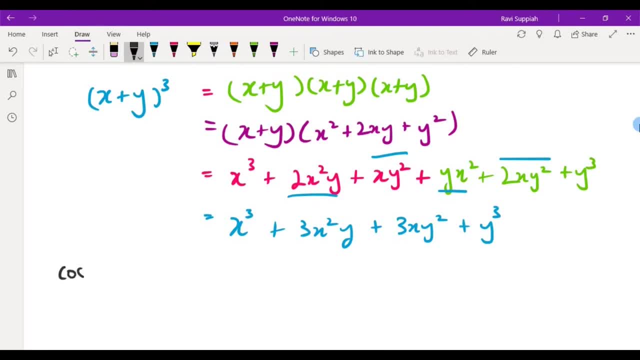 what you will get is cosine theta plus i sine theta cube. okay, cube is equals to, so x is cos theta, so this is cosine cube theta plus 3 x square y. so 3 x is cosine, so cosine square theta. dot i sine theta. okay, plus 3 x y square. 3. x is cosine theta and y is i sine theta, so i. 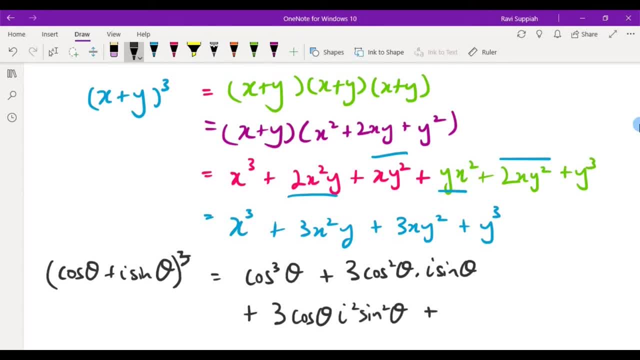 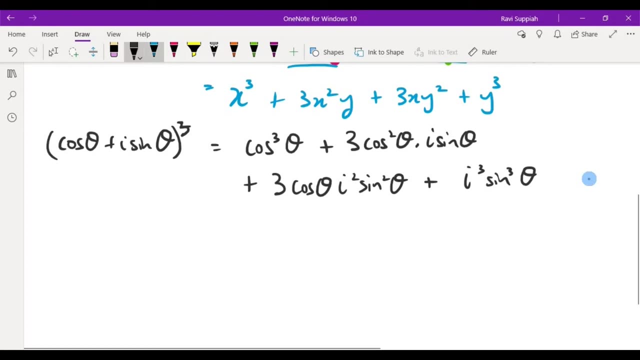 square sine square theta plus y cube, so it's i cube sine cube theta. okay, now what we can do is we can further see that i square is equals to minus 1. okay, so just quickly recap over here: i is actually square root of minus 1, so i square is equals to: 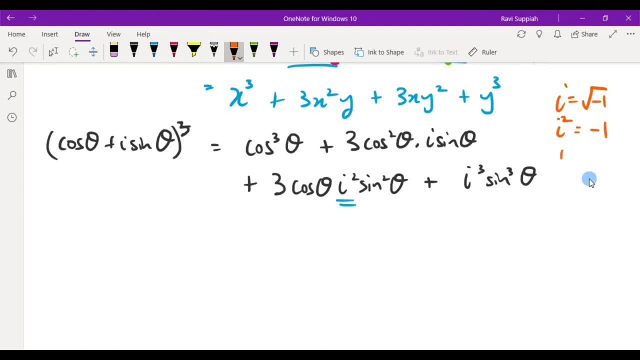 minus 1. okay, and i cube is equals to minus 1. is i square times i, which is minus square root of minus 1, which is equals to minus i? okay, so let's uh use this information to replace the i square and i cube that we 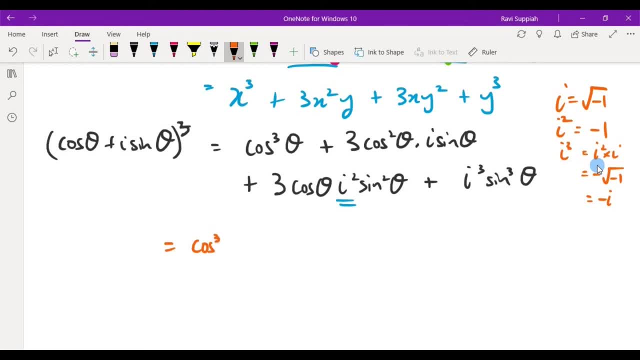 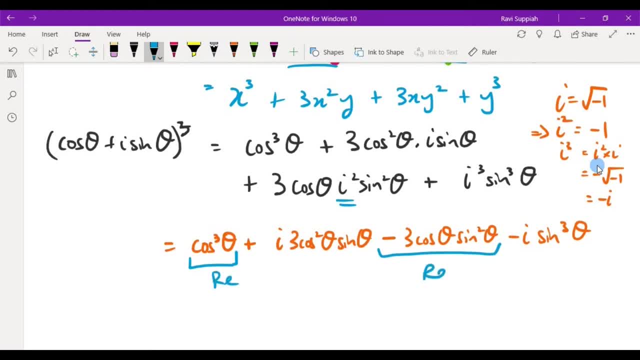 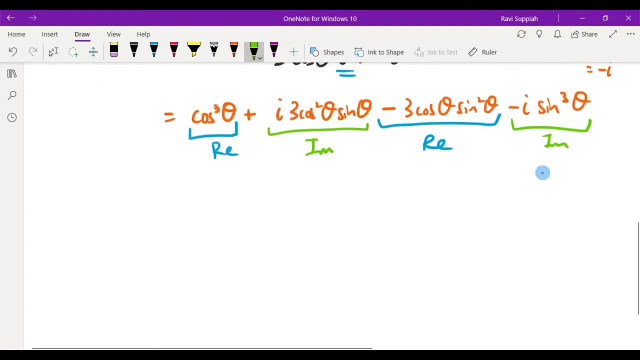 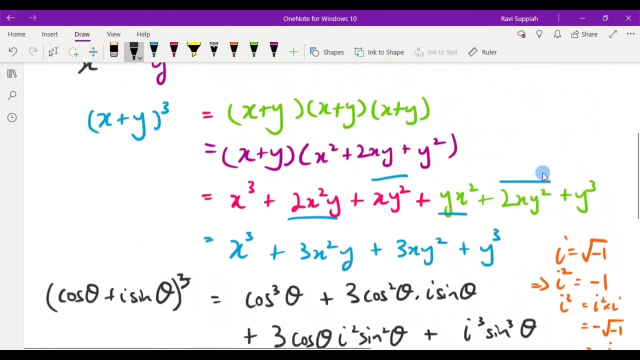 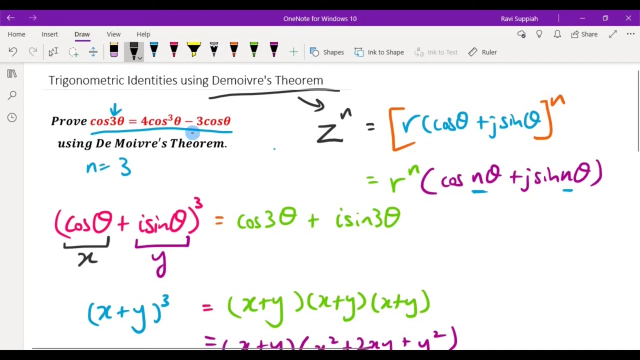 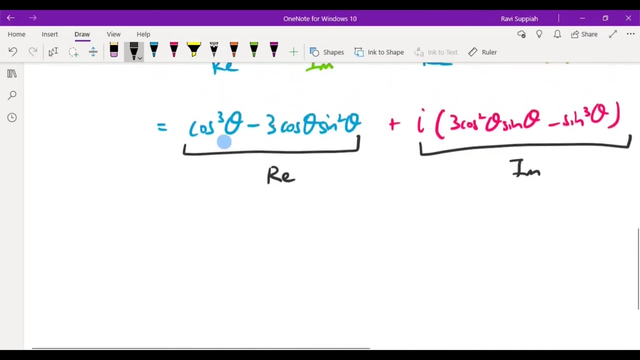 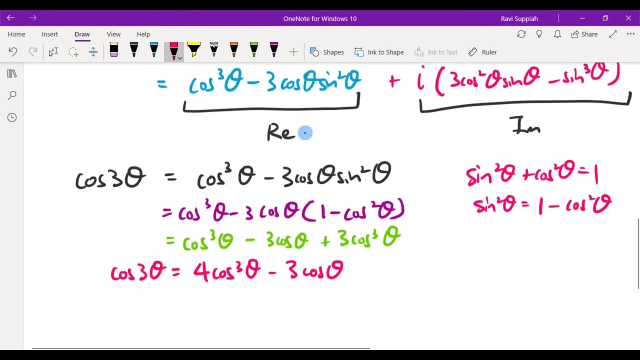